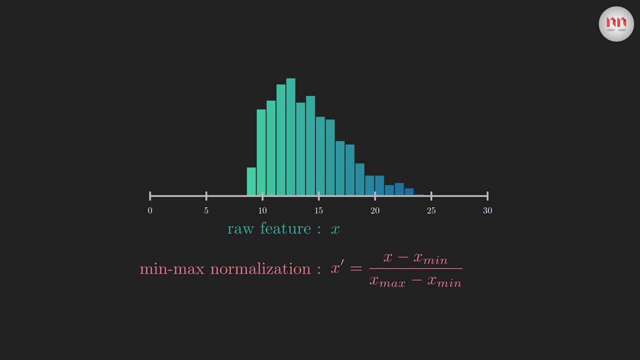 normalization. Let's see how it changes the data. Oh, it's too thin, Let's zoom in a bit. You can see that now the data lies between 0 and 1, and this is not a coincidence. Min-max normalization maps the data in the range 0 to 1.. Next comes 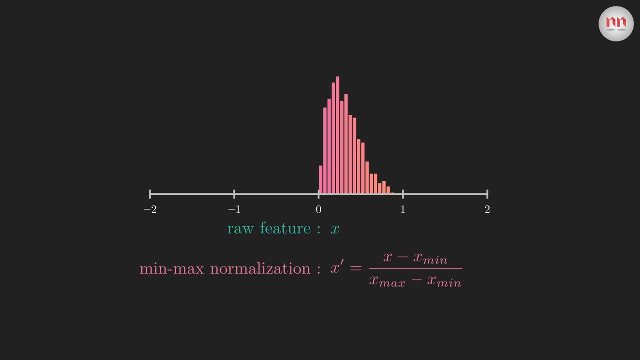 the most popular one, that is, standardization. Here we subtract x by its mean and divide by its standard deviation. After applying standardization, our histogram looks like this: Now there's a huge misconception among the beginners, that is, if we apply standardization, then it makes the 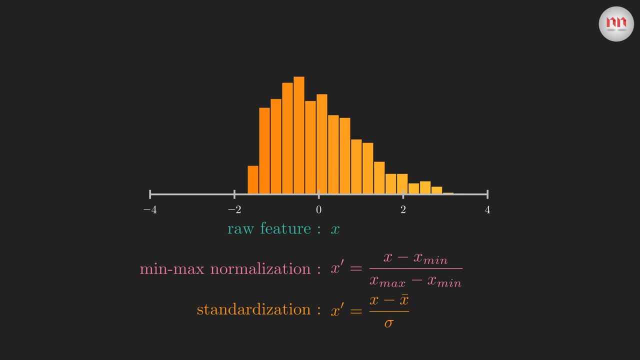 distribution a normal distribution. This is simply not true. Don't believe me. Let's take a very skew distribution. If we apply standardization on this distribution, you see the shape doesn't look like a normal distribution, does it? Well, the thing is, standardization is a. 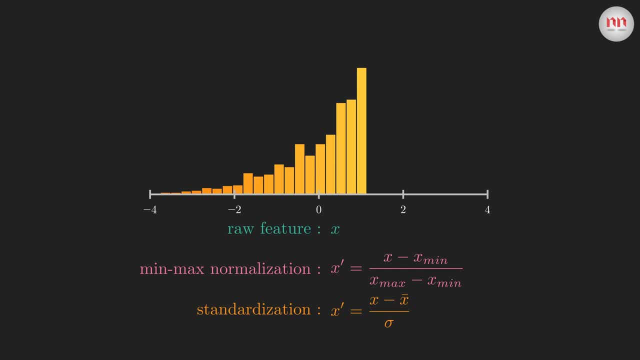 linear transformation. All it does is it makes the mean 0 and standard deviation 1.. If we want to change the general shape of our distribution, we need to apply non-linear transformations like logarithms, square roots etc. But I don't want to get 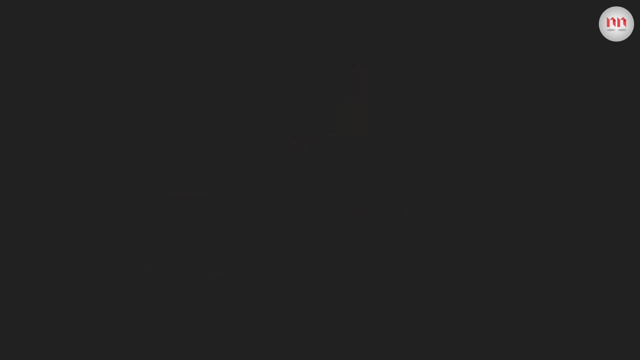 into those things today. Let's move on to the most important question: Why do we even care about feature scaling and normalization? Well, the first reason is to achieve faster convergence. Take the good old gradient descent algorithm. Assume that we have two features, x1 and x2 and theta1. 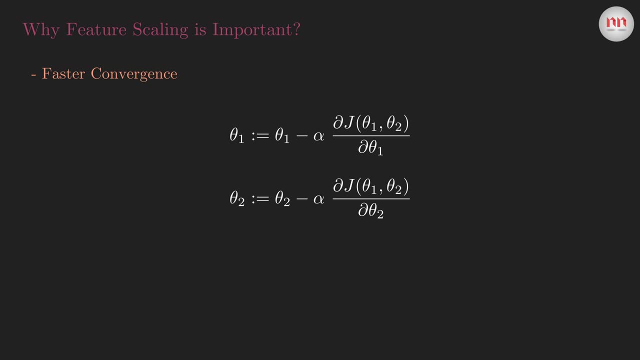 and theta2 are the corresponding weights. I'm ignoring the bias term here. If we assume the least square cost function, the weight update steps will look something like this: Now let's think of a scenario where we haven't done any feature scaling, Hence x1 and x2. 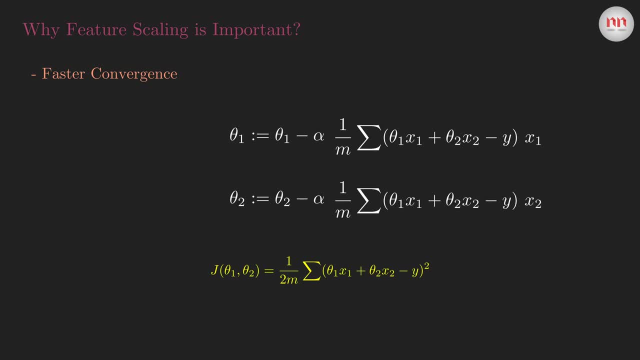 have vastly different ranges. Let's say x1 lies between 0 and 1 and the range of x2 is 100 to 1000.. So what do you think will happen during gradient descent Due to the small value of x1, the